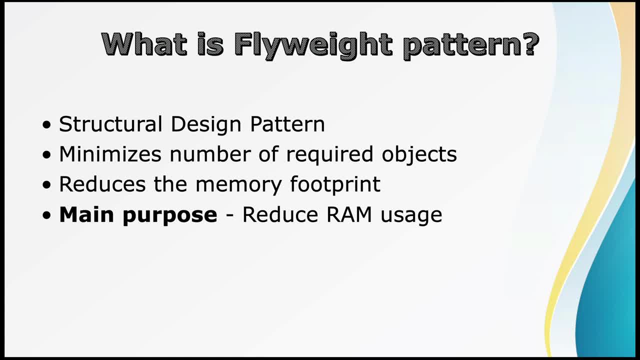 design pattern. So it's a structural design pattern and main purpose of this design pattern is to reduce the memory usage by reducing the number of required objects of the program. So to understand this behavior of this pattern, let's look at the example and then we will. 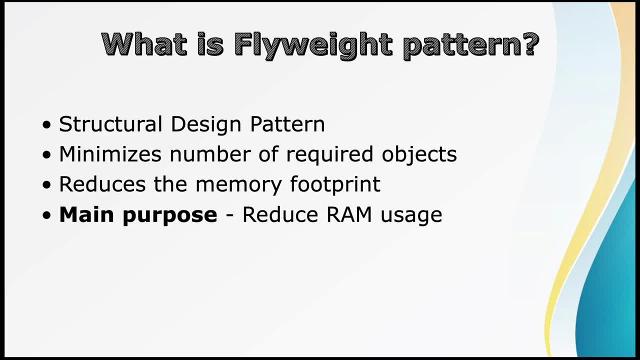 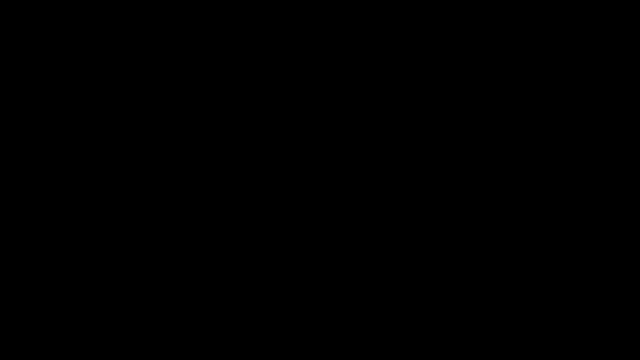 discuss about what are the benefits and drawbacks of this particular design pattern. So we are going to start with a bug. So this is a bug that we already have in Python. The bug is that it produces a number of elements, So it is an object that stores the number. 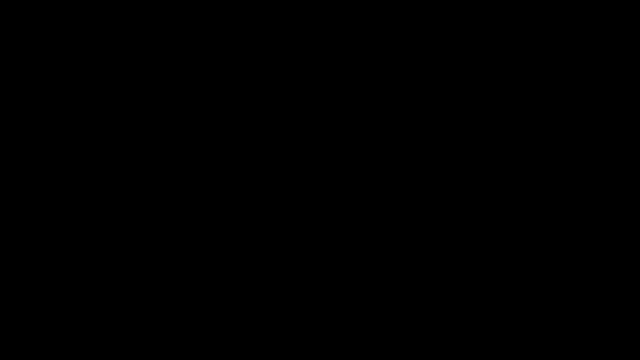 of elements in the program, And this object is a number. there are three elements in the program. The first element is a number, because it stores the number of elements of the program. And the second element is a number because it stores the number of elements And the 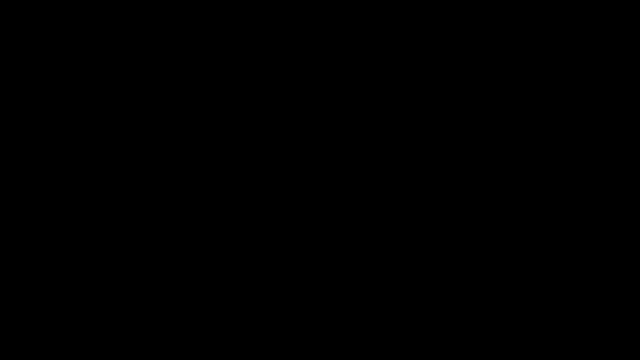 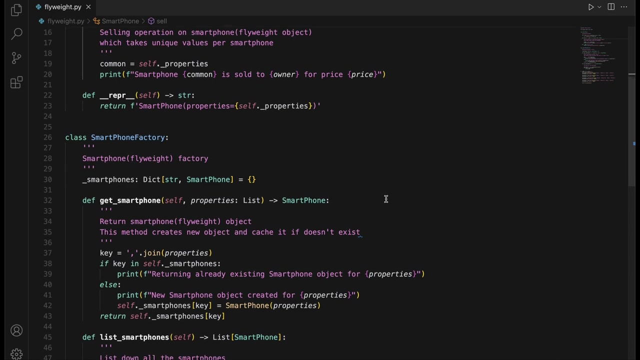 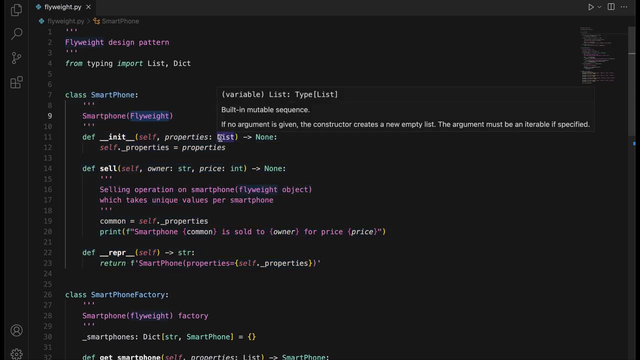 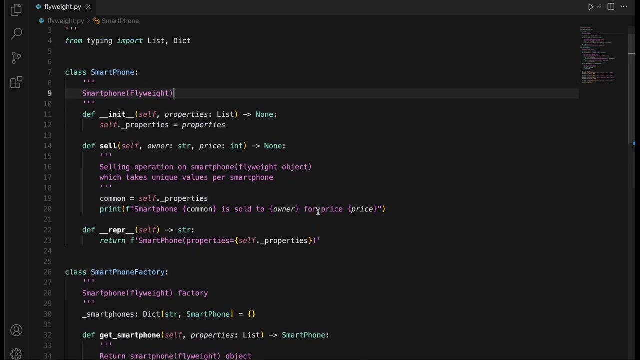 So this is the example where I have taken example of smartphone factory, where you will have a smartphone class which is nothing but a flyweight class, and so how this pattern is being implemented actually. So what you need here, that is as much as possible. you have to share the properties or share. 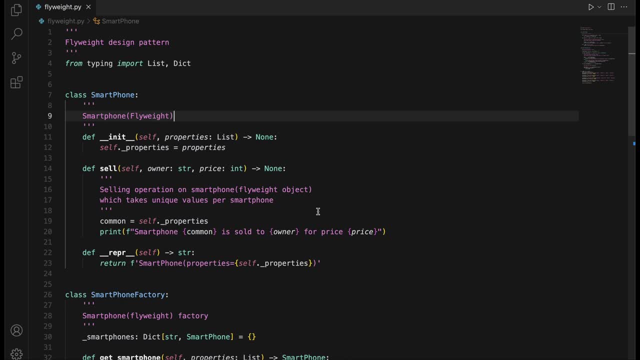 the memory, So that way you can reduce the usage of memory. and to do that, what you will do? you will make common properties for specific object and you will keep it as it is, and whenever you need something complex, you will use that particular common thing and then you will add additional. 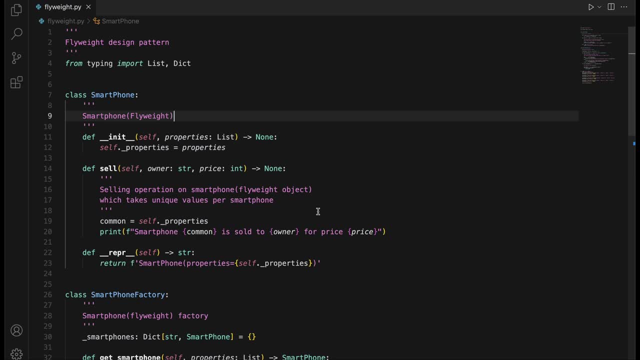 on top of that. So if you remember, I mean there are lot of examples in real life as well, Like suppose you take an example of any food outlet where they keep some few things ready, right, and whenever they need to make something complex they will use those common things. 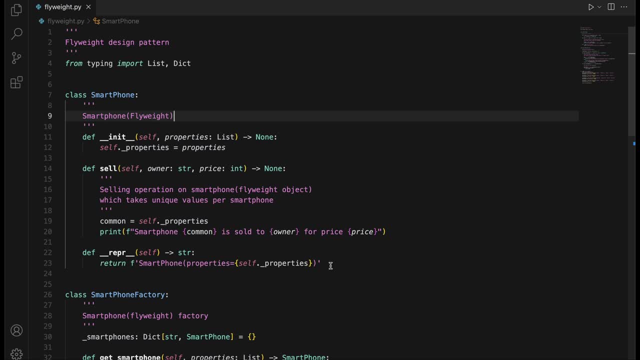 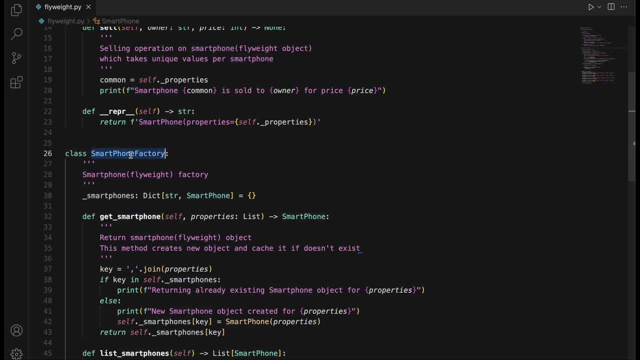 and then make it right. So that is how they reduce their work, The same way. we have taken example of smartphone here. this is smartphone factory. So let's look at the implementation of these two classes and then we will understand how it works okay. 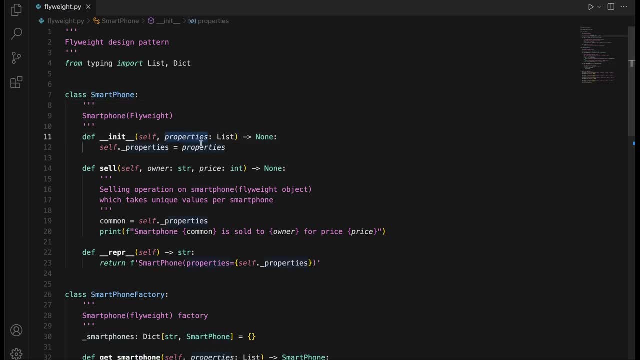 So here is the class smartphone Which takes the properties and you set it private property private. what can I say? it's yeah, again, it's a property right. So whatever information you give for this smartphone, this will be set here in self dot underscore properties. okay. 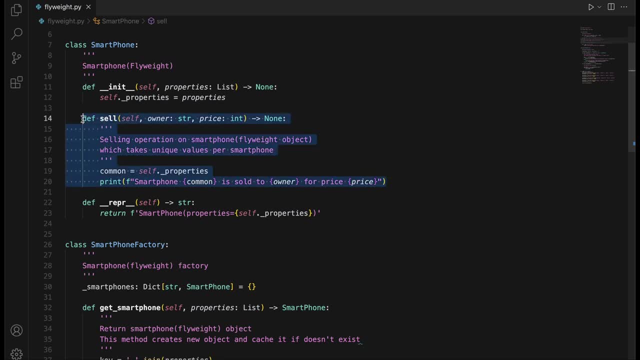 And this is the operation function, basically, whenever you want to add something- suppose you can take an example of preparing a recipe. right, and while preparing the recipe you will use some common things And then you will add which is unique for the particular recipe, the same way for any. 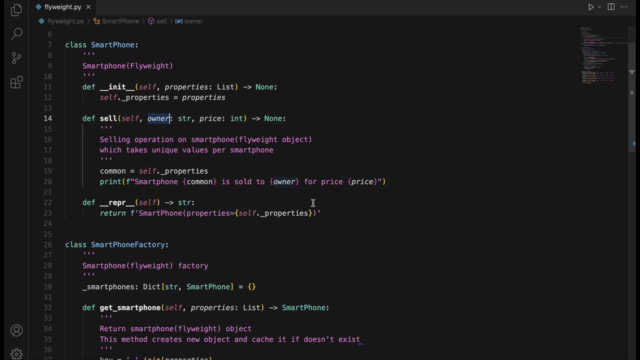 specific smartphone, what you need. suppose we are selling the smartphones here, So what will be the unique? you will have all the models common, but owner will be different and price will be different in all the cases, right? So that is why we are taking this owner and price here. these are additional information. 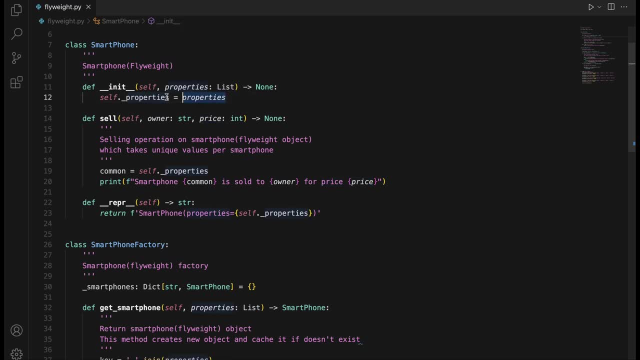 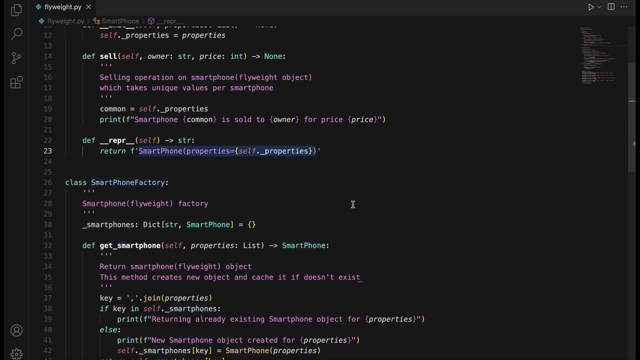 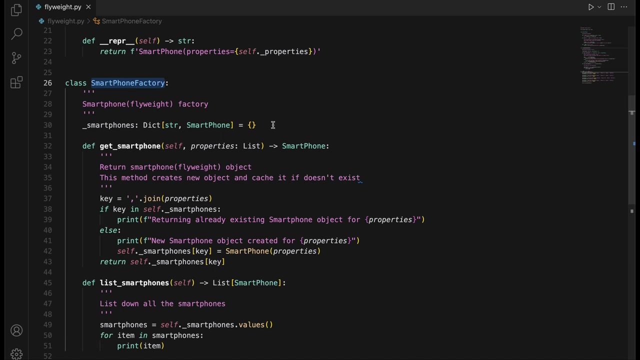 for the smartphone. but what are the common parameters? are there which are already set? So that is smartphone object. and this is just a representation method. and let's look at the factory method now: factory class, So what factory class does? So, basically, how we reutilize these classes or objects. 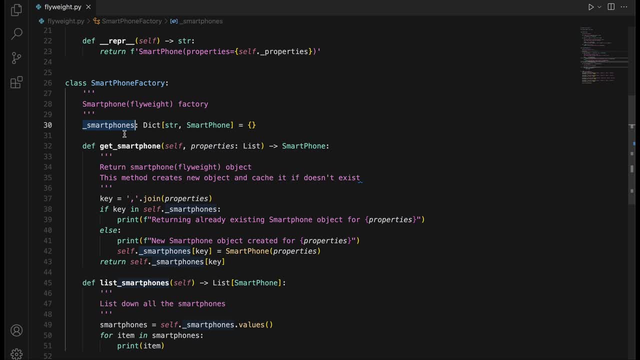 So basically we create one class property here, okay, And that is dictionary of key and value as a smartphones object. So we will store here based on properties. So suppose properties are. there is like let's take an example of iPhone 14.. So there are three properties we are mentioning here. 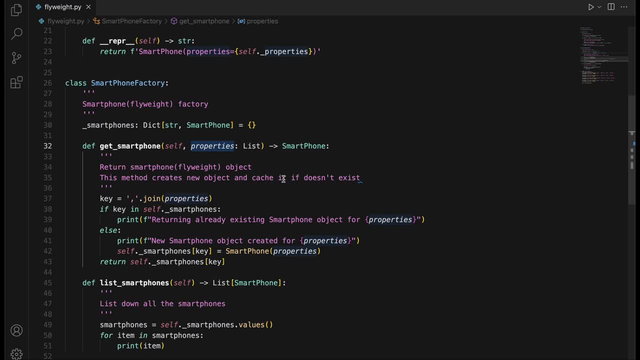 Apple is a brand name, then iPhone 14 is the second property, Then third property is suppose it's a color of that. or maybe fourth property is a size of the memory of that particular smartphone, So suppose 128 GB. So those properties you have sent here, and when you try to do that you will create you. 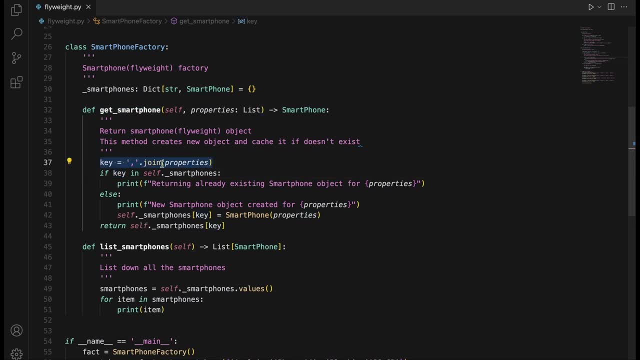 will first check. First of all, you will create a key based on those properties. So suppose those four properties are there, right? So I'm just what I'm doing here. I'm just joining by comma, or you can. you can do also like this hyphen: okay. 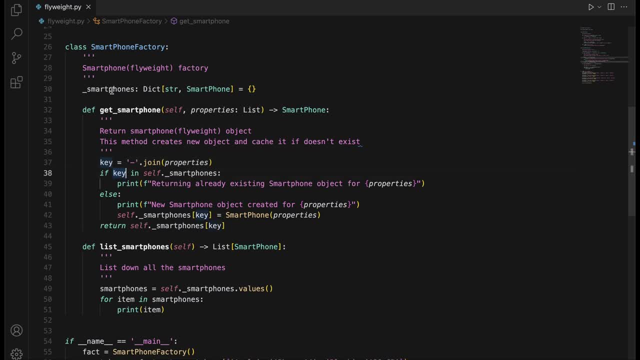 So, once that is done, you will check that key in this smartphones dictionary. if it is there, then we are printing that returning already existing smartphone object for this properties or with this properties. Else, if doesn't exist, Then what you will do? You will create an object of the smartphone which is nothing but this. fly with class and 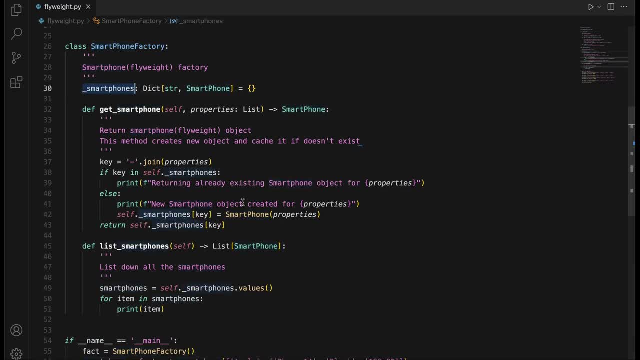 you will add that instance in particular dictionary. So next time, whenever someone tries to get the similar smartphone- iPhone 14- with black color, then you will get the same response: same object, but not. you're not going to create the separate memory for that. So that is how you are going to reutilize the memory. 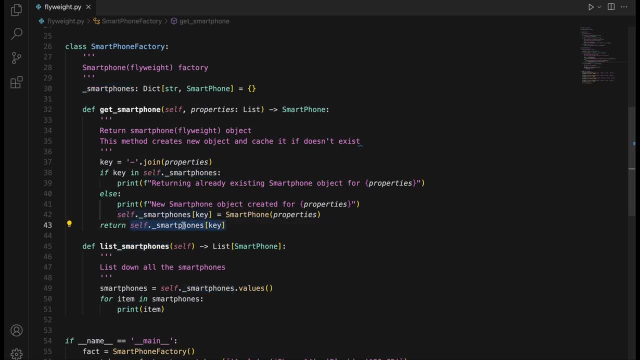 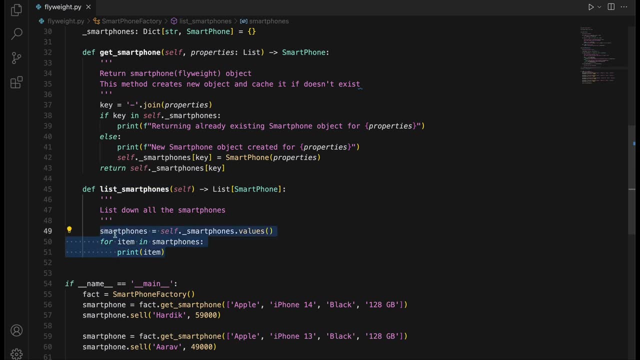 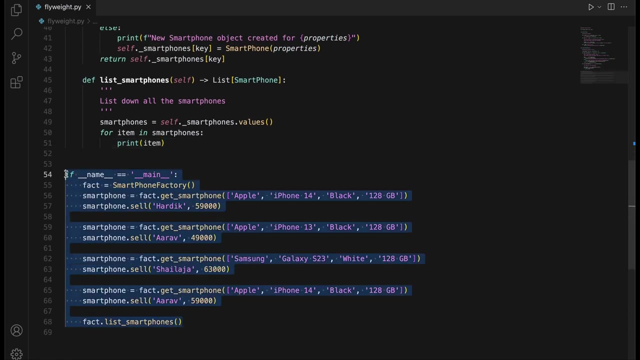 Okay, So. So this is how you will return the object of this smartphone. Now, this is just a extra method where you will see how many smartphone objects are created. Okay, So we will check that Now, once we run this, how we can check that it is working properly. 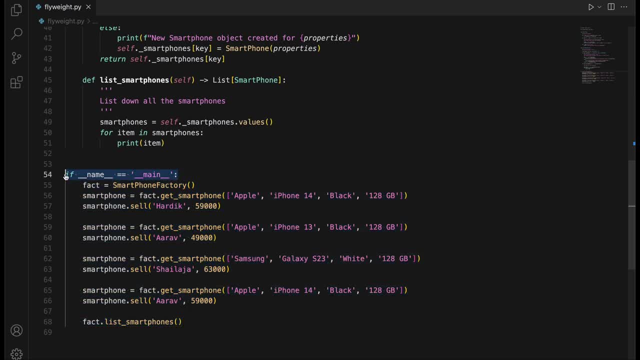 So look at this. what can I say? it's a boiler pit floor running module as a script. So I am creating one instance of this factory, Okay, And I'm trying to get this smartphone using these properties: Apple iPhone 14, black and 128 GB. 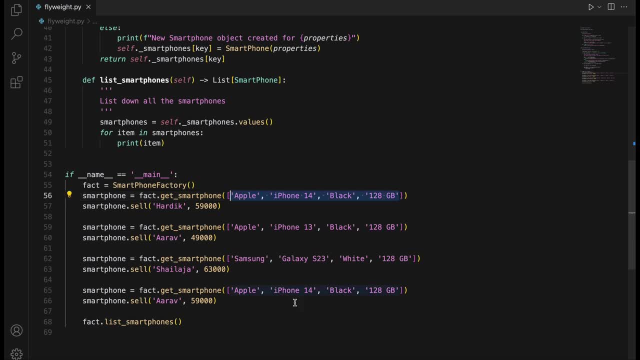 So if you see here, these all properties are also used in this fourth request. Okay, So first three requests are having separate instances of smartphone because all have different properties, Right? So here I am calling this cat smartphone. I'll get that And I will try to sell it to Hardik with this price. 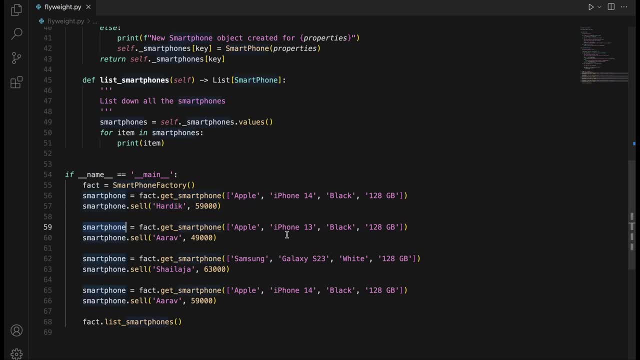 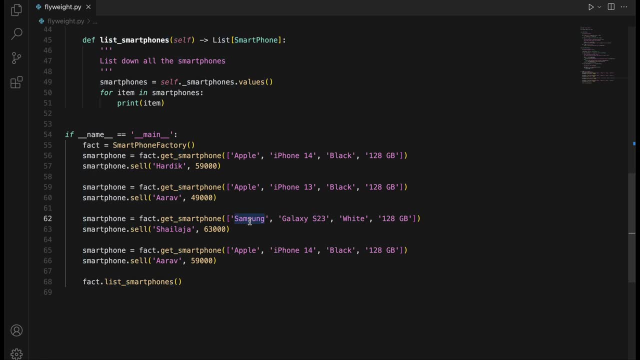 Okay, Then again I am getting the smartphone, which is iPhone 13, then 49,000 and arrow Again. this is third smartphone. again it's a separate smartphone. But now what I am doing here? that arrow is coming back and wants to buy iPhone 14.. 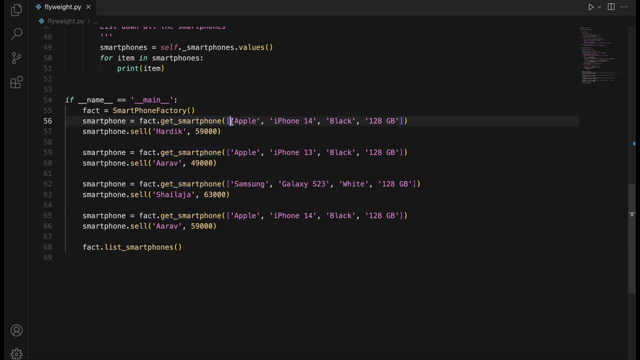 So you are what you're doing here. we are trying to get smartphone with the same properties And this time, actually, you should not be creating a new object, because you have that object available already in memory. So to reutilize that, what you will do? you will try to get the same object and try to. 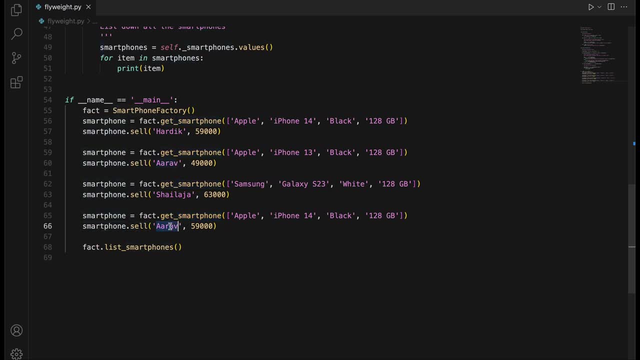 sell it. Okay, So smartphonesell. and then this time I am just changing this thing and value is same because phone is same, Right. And now, if I will try to list smartphones in case of other design pattern or normal program, what you will have is four objects of the smartphones, but here, as we have used, 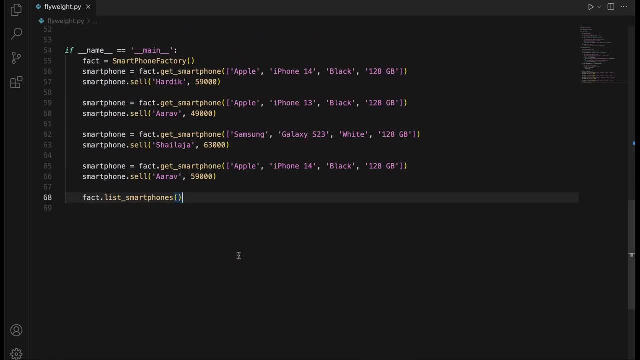 this pattern- flyweight pattern- where we are reutilizing the objects. Okay, So after reutilizing the objects, you will be able to see only three objects, because this is reutilized version. Okay, So now let's run the program and we will understand how it works. 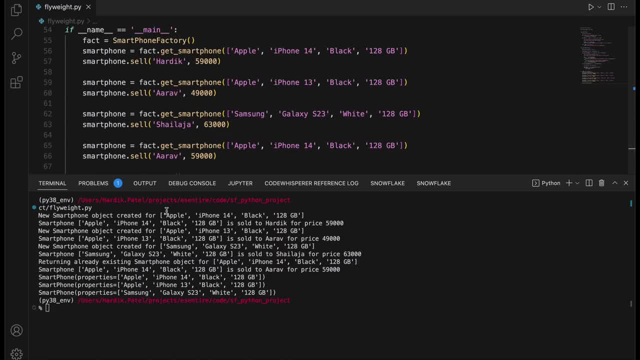 Okay, So, as you can see, first time it was created and was sold to Hardik, with this price, again created. second time, it was sold to Arav and this price. third time, also it created, but the fourth time when I tried to get the same smartphone which was created earlier. 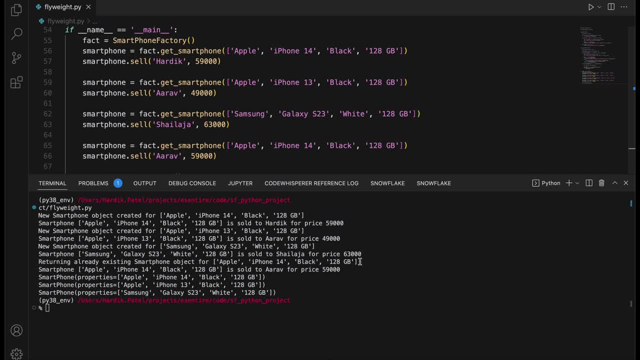 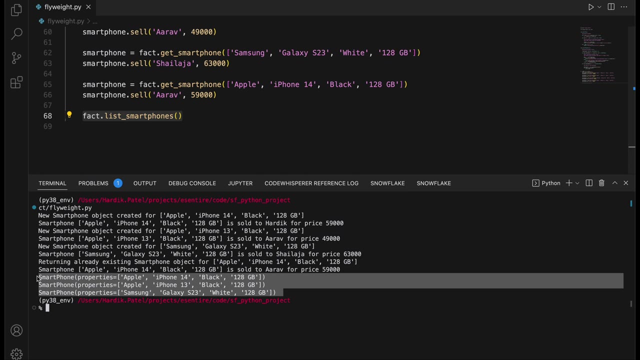 This time it is returning already existing smartphone object for this properties and the same smartphone I am selling to Arav with this price. Okay, So that way. and now the last statement of this program, that is, listing out smartphones. So basically, we have only three smartphones. 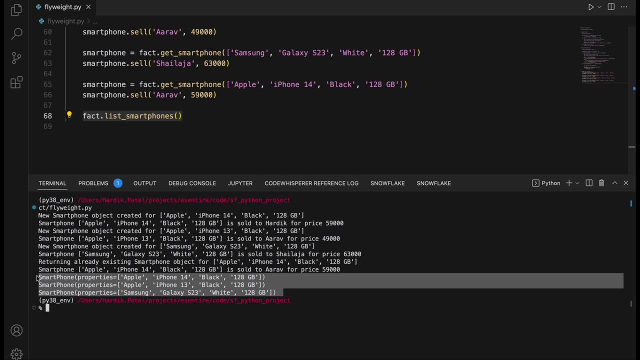 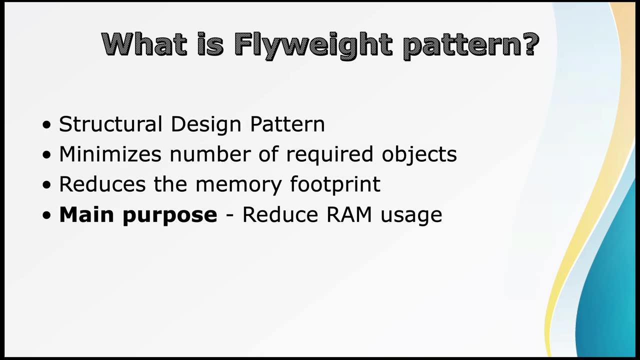 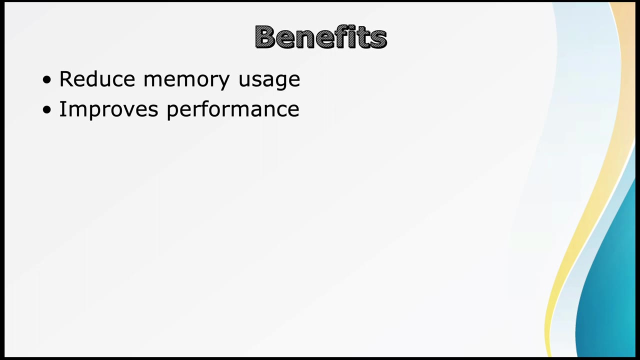 That means three objects only. So basically, we are saving the memory here. Okay, Now let's look at the benefits of this pattern. So what are the? yeah, as we already mentioned that it tries to reduce the memory uses, Okay. So major benefit of this pattern is that you will end up using less memory in your program. 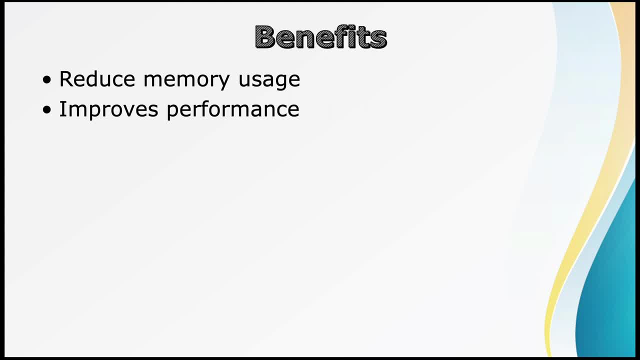 which will increase efficiency of the program and hence you will get additional benefit of performance improvement, right? So those are the benefits of this design pattern. Now let's talk about drawbacks. So drawbacks is just a simple one, That is, complexity. Okay. 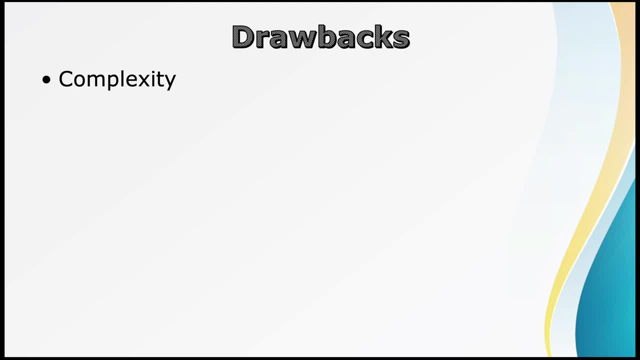 And mostly you will end up making complex code and that will be more complex for new developers to understand, right. So this is one of the drawback and so, based on this drawbacks and benefits, I would conclude that, until you do not foresee any memory issue in your program, you should avoid this pattern.